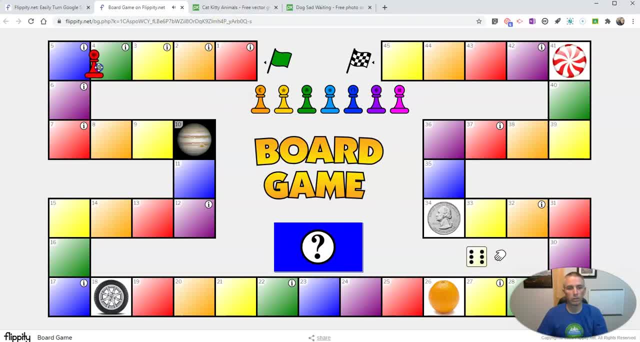 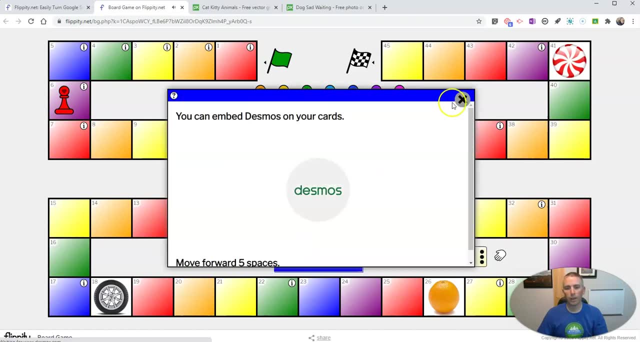 three dice to roll, So I'll move this person's marker six spaces forward and they can then look at what their card or what their space says. Now we also have cards that you can draw, And these cards again will pop up with different pieces of information. 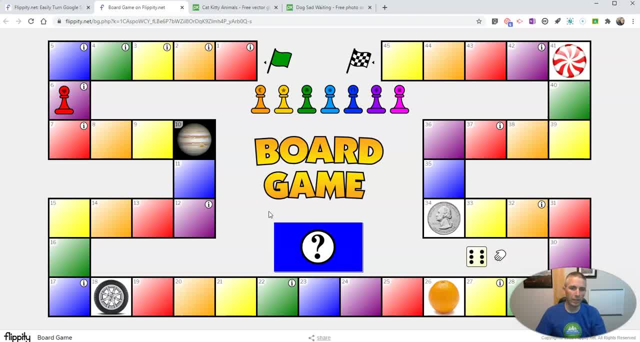 And there's a lot of flexibility with what you can do in those cards and in these messages that you have up here on the spaces. You could have students try to answer questions. You can include fun trivia facts. You could have students move forward or backwards depending on what pops. 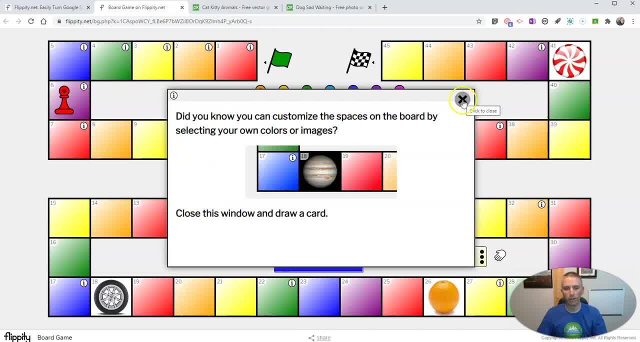 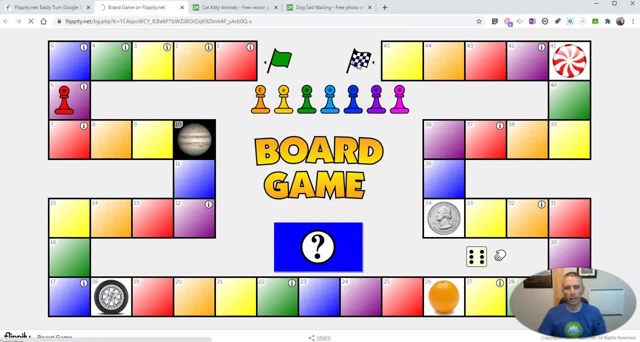 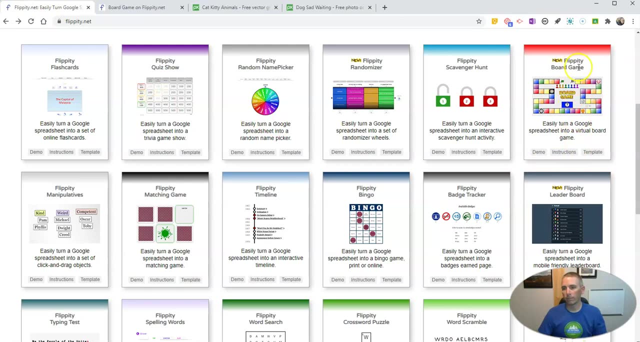 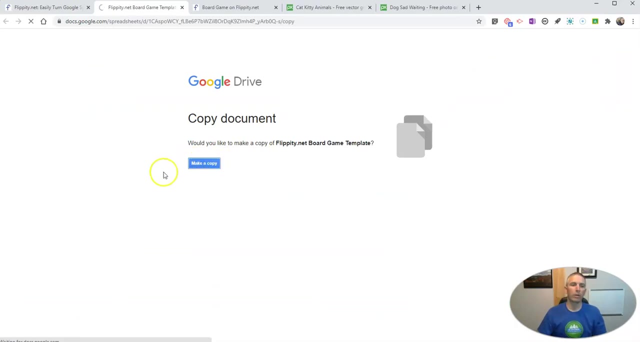 up on the card or in the bit of information. So let's go ahead and take a look at how you can now customize this game and make it your own. So go to flippitynet and choose the Flippity board game and click on template and you're going to make a copy right into your Google Drive or your Google. 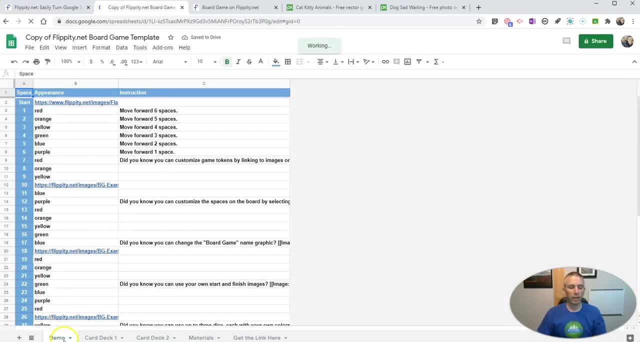 spreadsheets And when this loads, we'll see down here in the demo field. This is setting up our game board appearance 1MATCHÁTCOM. you can't edit anything that's in blue, So don't change anything that's in the blue. 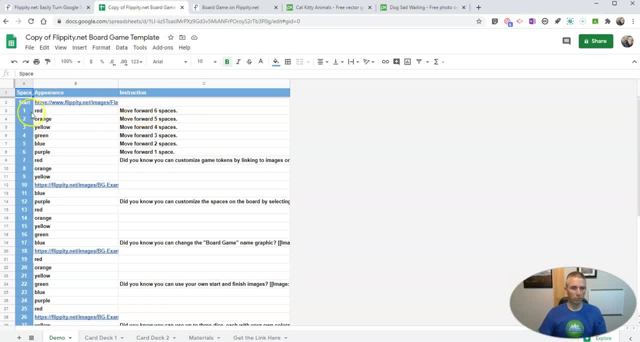 but you can change everything else. So if you want space number one to say something instead of move forward six spaces, it could be something like fun fact. The Red Sox have won the World Series three times this century, And over here we can do. 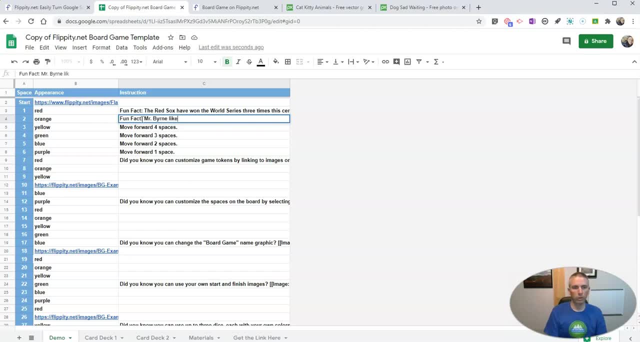 fun fact: Mr Byrne likes to ride his bike. But you can also do things like go and do, things like go back three spaces, Or you could do a little challenge Like move forward seven spaces If you can hold your breath for seven seconds, So you can have fun with it. 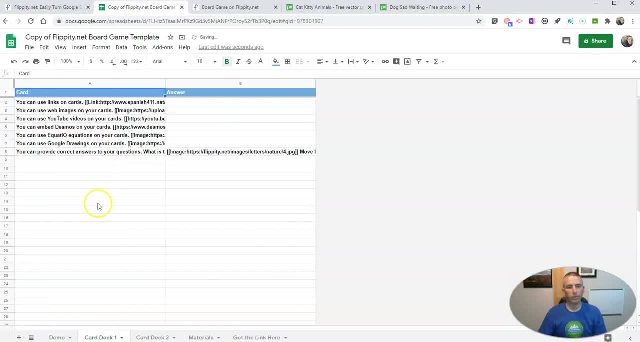 Now here in our cards, you can link to anything, just about anything you like, including a website, a YouTube video, an image or- you'll see here Desmos and Google Drawings- links can be included. So if you want to include a link to a graph or a link to an equation, 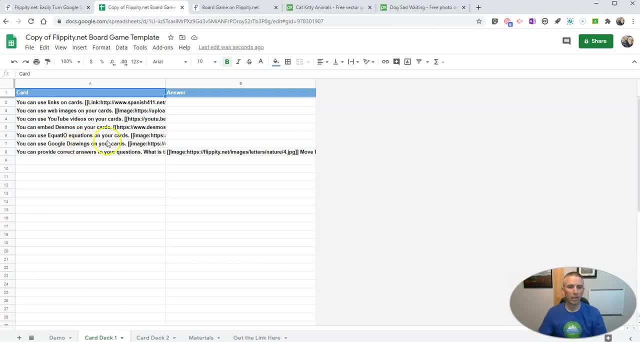 you can do so, or any drawing you created with Google Drawings you can link right in here. And, of course, you can write anything you'd like as well. Right, You won the spell, Mr Byrne spelling bee. Then say: move forward 10 spaces Again. I can link into just about anything. 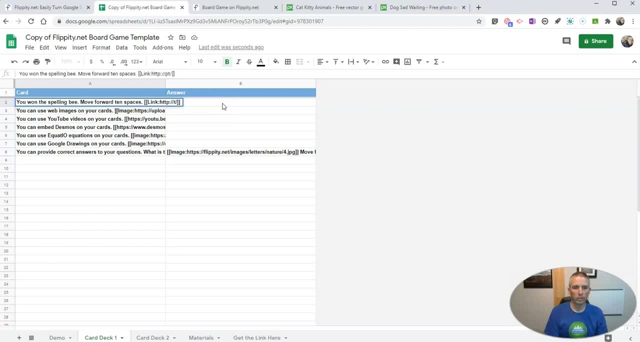 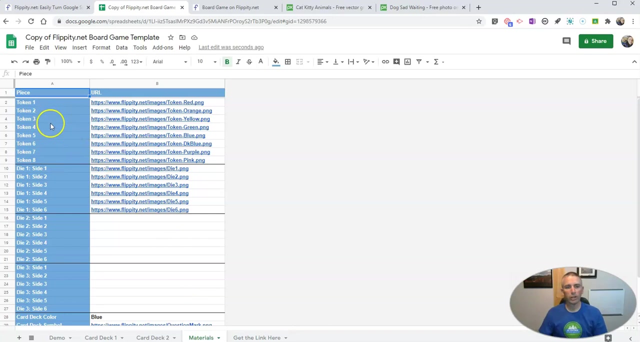 in here. Maybe I'll do something like link to the ABC spelling games. It's, I'll put that link right in there. Now you can have two decks of cards, So you can have a whole another column here of up to 45 cards In the materials section. this is where you can change your. 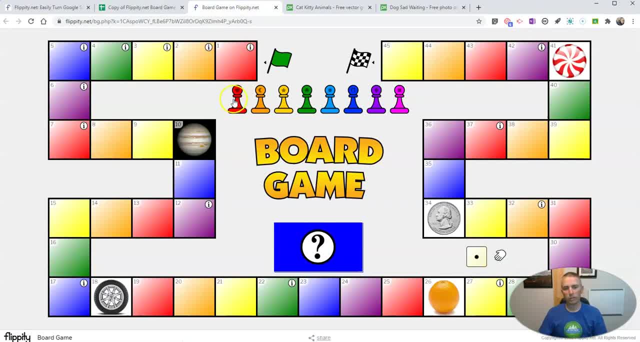 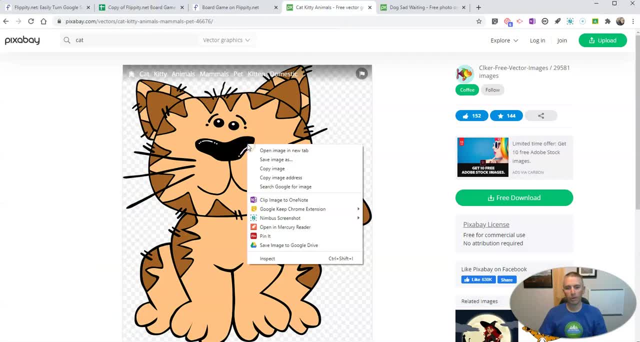 game tokens or your markers. So instead of using just these standard ones that Flippity includes for you, you could do something like include a picture of a cat. So I'm going to use this picture of a cat. I'm going to copy the image address. 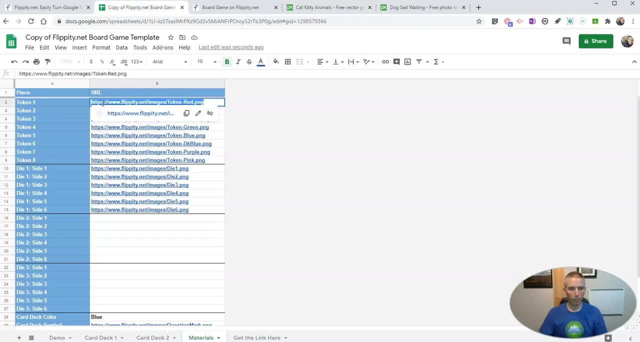 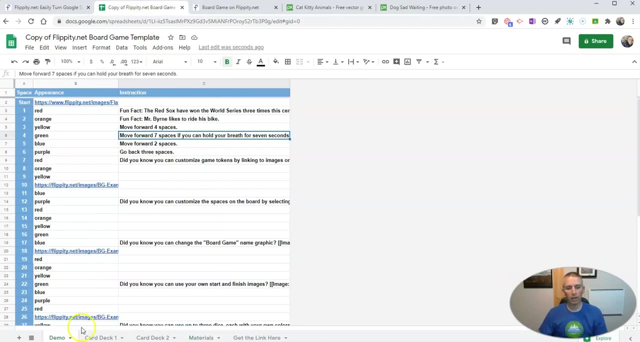 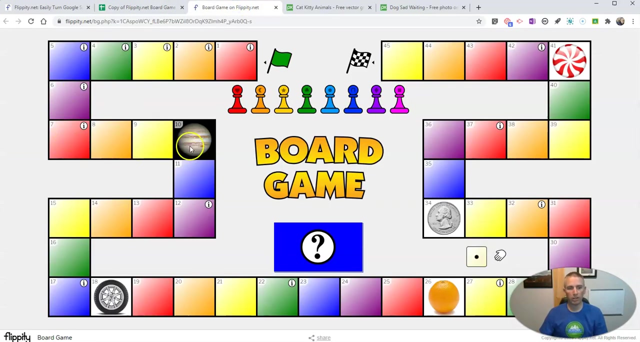 And I'll put it in here for my token one. And so now I have a cat instead of that standard red marker When I'm done setting up my game, and I have all the pieces that I like and I have all the cards that I like and, by the way, you can have each one of these spaces. 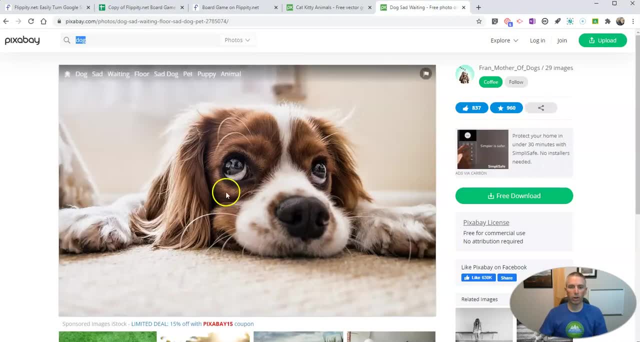 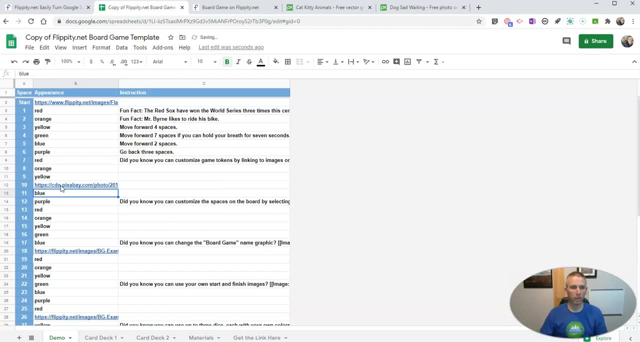 include a different picture if you want to. you know, if I wanted to include a dog, copy that in there. So I'm going to use this image address And I'll put in a picture of a dog for space number 10.. When I have it all set up the way that I like, I have to go to the file button and publish.